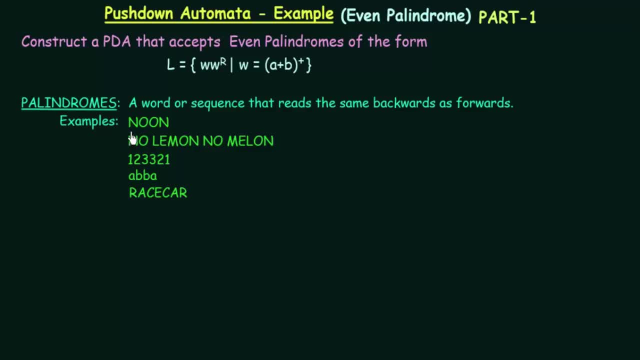 For example, I have some words here from English like noon n-o-o-n. If you read it from the front it is n-o-o-n and from the back side it is still n-o-o-n. And here I have another sentence which says: no lemon, no melon. 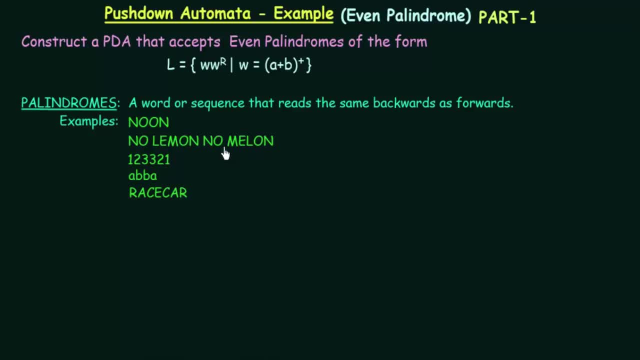 And if you read it from the back word, it is still: no lemon, no melon. It is the same. And we can also have numbers like this: 1, 2, 3, 3, 2, 1.. 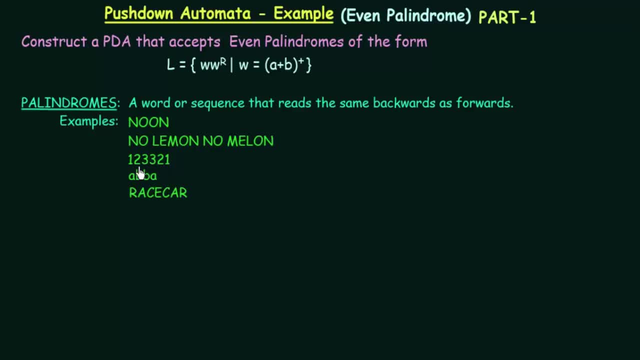 And if you read it from backwards, it is still 1, 2, 3, 3, 2, 1.. Or we can have sequences like this: A, B, B A. From backwards also, it is A, B, B A. 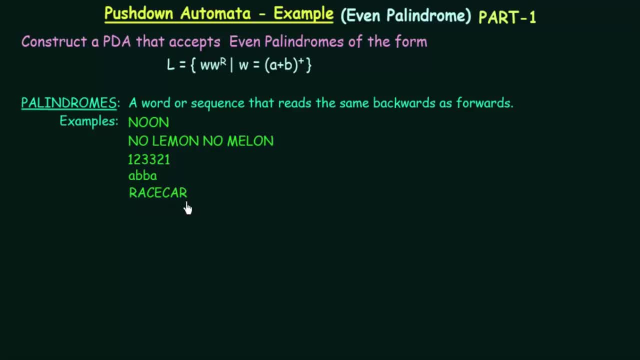 And here I have another word which says race car. If you read it from backwards also, it is still R-A-C-E-C-A-R race car. So these are examples of palindromes, And we want to construct a push-down automata that accepts even palindromes. 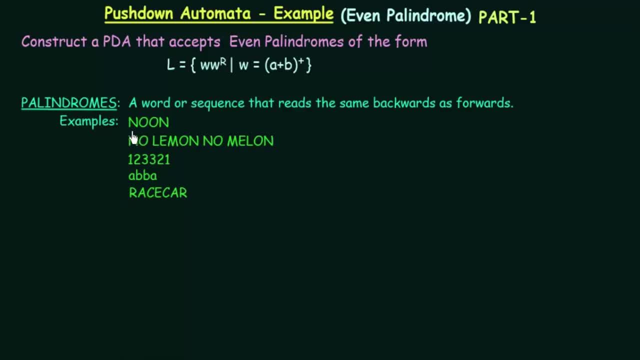 So here, from the examples that I have shown you here, these words like noon, four letters, and even this sentence, it has 14 letters, it is even, And even this number, it has six digits, which is also even. 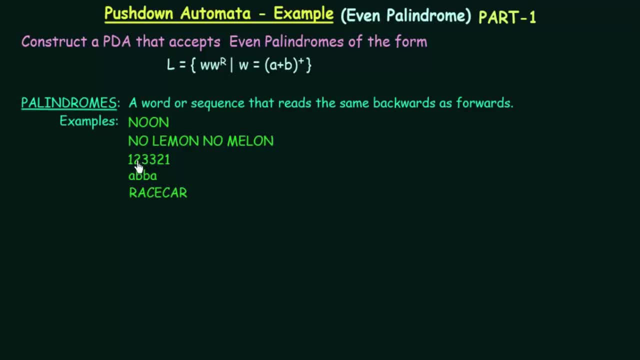 This is also having four letters, which is even. So. these kind of things are what we are going to design, But this race car it has seven letters. It is not an even palindrome, it is an odd palindrome. So we want to design PDA that accepts even palindromes. 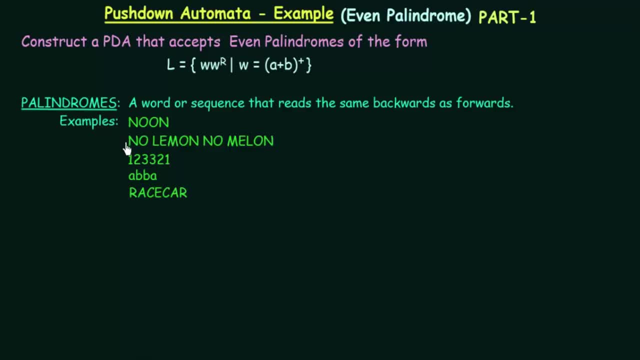 But we are not going to design palindromes that accepts all these letters like this. our palindrome is limited to only A and B, the symbols A and B. The palindrome should contain only symbols A and B. And what do we mean by this? positive closure. 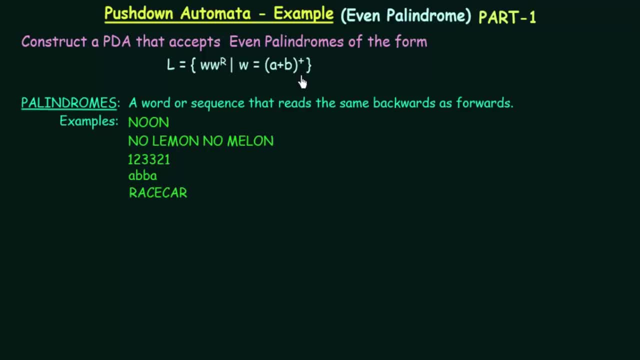 Positive closure. if you remember when we studied about regular expressions, I have taught you: if you see positive closure, it means that it should contain at least one symbol and it cannot be empty. Epsilon is not allowed, But if you see a star symbol over here, that means it also includes the empty symbol. 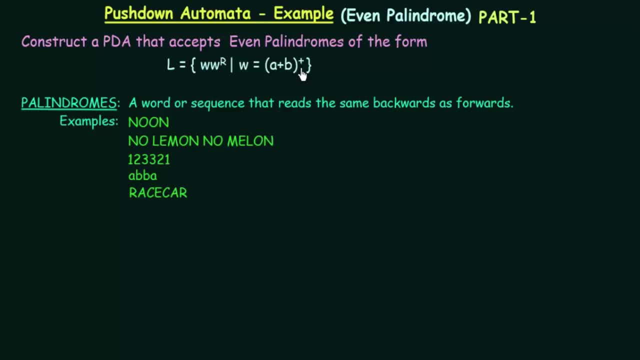 But since we have a positive closure or a plus sign, it means that it cannot be empty. at least one symbol should be there. And let us see what the meaning of this language is: W. and then we have WR, which means the reverse of W. 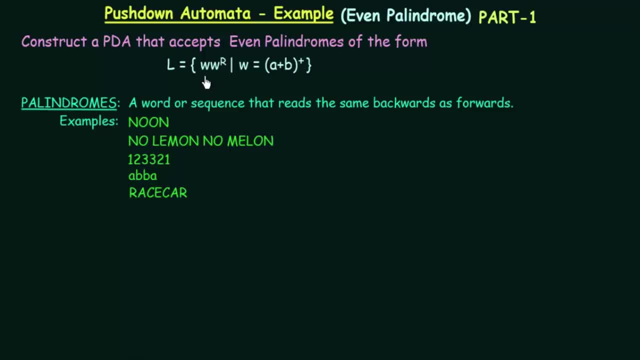 First we have W, which represents the first half of the string. For example, if you see this word N O O N, the first half is this one: N O. this represents W And then W superscript R. this represents the reverse of the first W, which is O N. 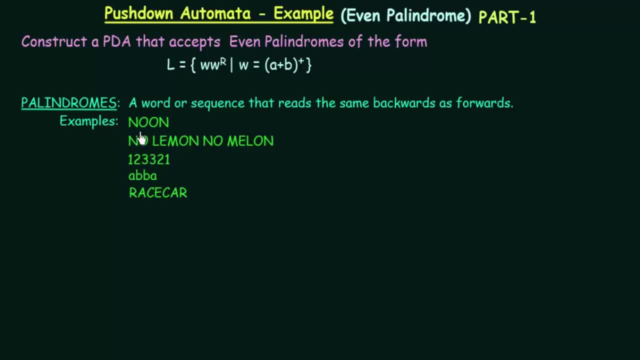 N? O is the first W and then O? N is the reverse of the first W, which was N? O. So this is how you denote a palindrome in this kind of language representation, And now we have to design the push down automata for this. 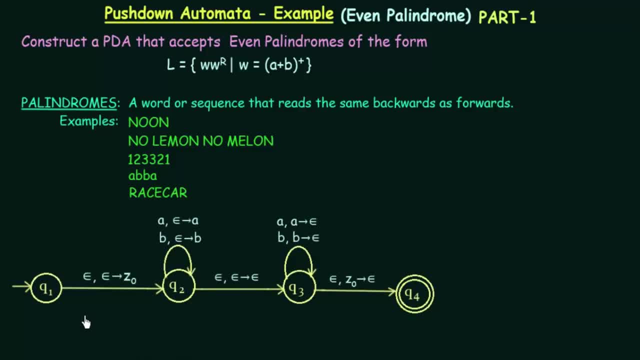 And let us see how we can do that. So here I have already drawn the push down automata for this, And here we have four states And we start with the starting state, which is Q1.. And in Q1, let us see what happens. 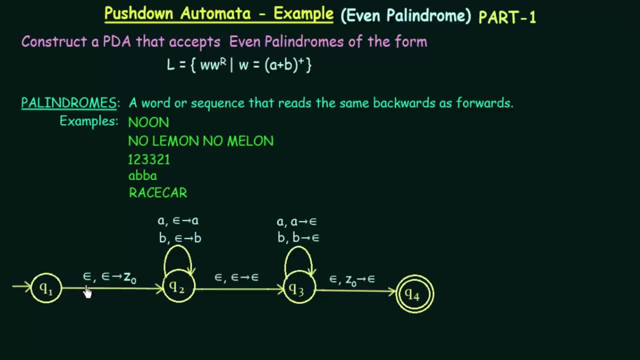 We don't read any input symbol- it is epsilon- And we don't pop anything from the stack, But we push a symbol Z0 to the stack in order to denote the first element of our stack. So I already taught you that in push down automata we always have a stack. 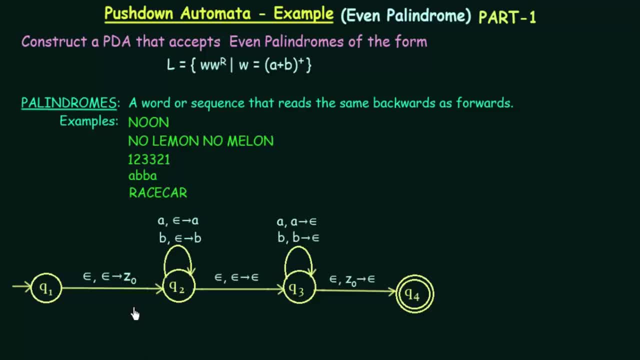 And then we always want to know what is the bottom most element or the first element of the stack, So that we can know when we reach the end of the stack. So I hope you know what these symbols mean. If you don't know, I request you to watch the previous lecture. 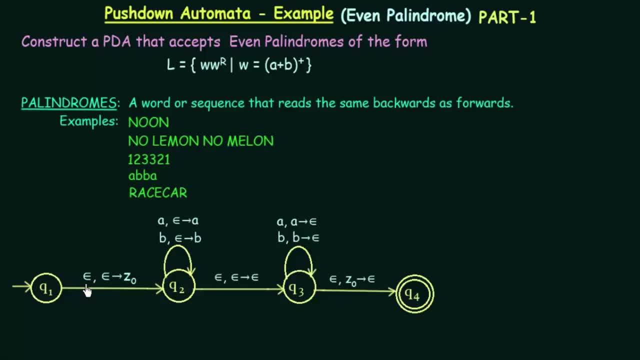 So here in state Q1, we are not reading any input symbol And we are not popping anything from the stack, But we are pushing the element or symbol Z0 to the stack in order to denote the first element of the stack. Then we come to state Q2.. 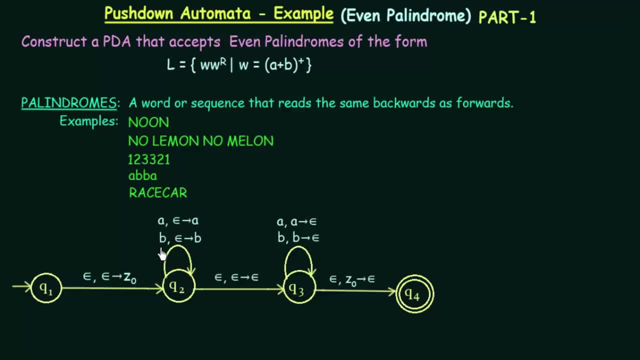 In Q2, we can either get input A or input B. Now if we get input A, we don't pop anything from the stack, but we push that A to the stack, And by pushing I mean inserting. So if we get input A, we just push it or insert it to the stack and we don't pop anything. 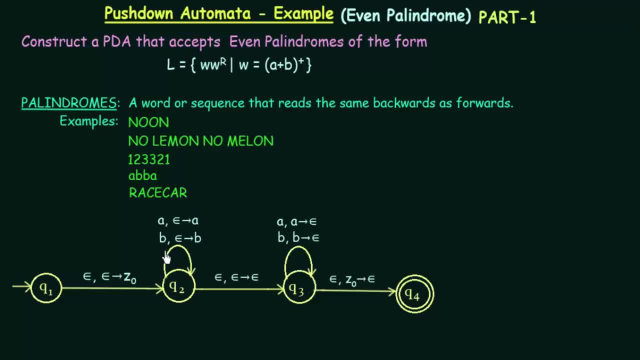 And in the same way, if you get an input B, then what we do We just don't pop anything from the stack, but we just push that B directly into the stack. That is what we do in state Q2.. So at this point we assume that we have reached the midpoint of our string. 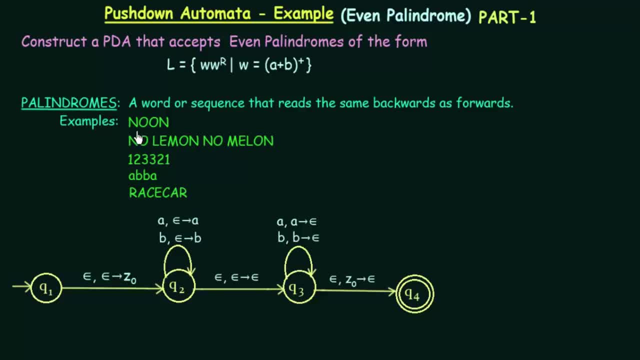 Like, for example, if we were taking this: we assume that we have completed this, NO, and we are reaching this middle point. So when we reach the middle point, what we do? We don't read any input symbol, We don't pop any symbol. 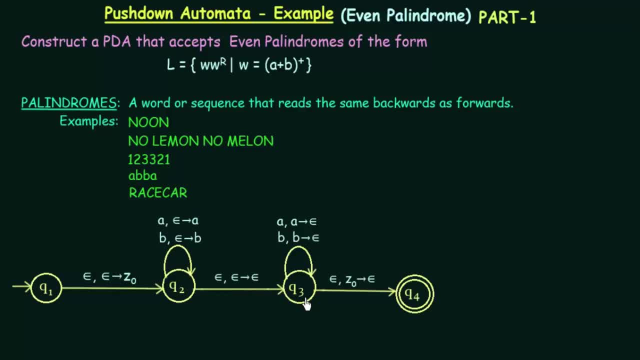 And we don't push any symbol, But we directly go to the next state, which is state Q3. And in state Q3 also we can get inputs either A or B. And let's see what we do If you get input A. 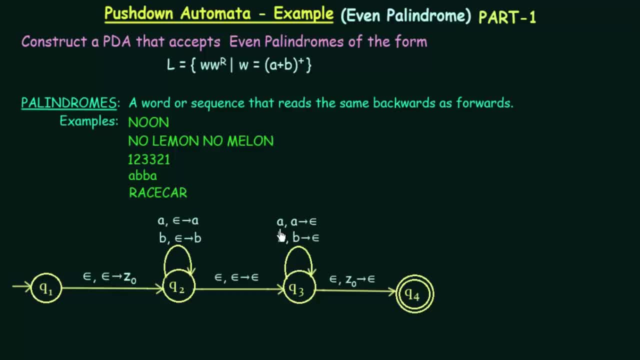 you pop A from the stack and don't push anything. So if you get an A, you check if A is on the topmost of our stack or not, And if it is there, then you pop it and don't push anything. 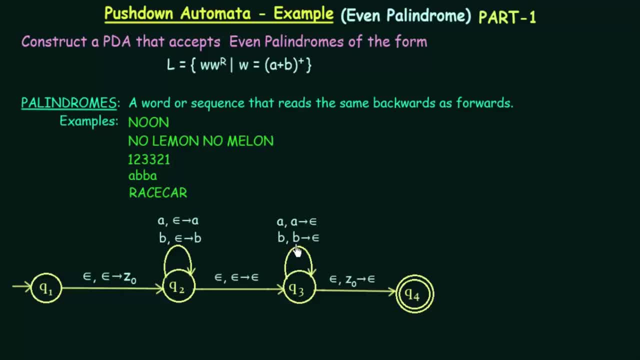 And similarly, if you get B again, you check if B is on the topmost of the stack And if it is, pop it and don't push anything. So this is repeated until our string is fully consumed or still our string is finished. 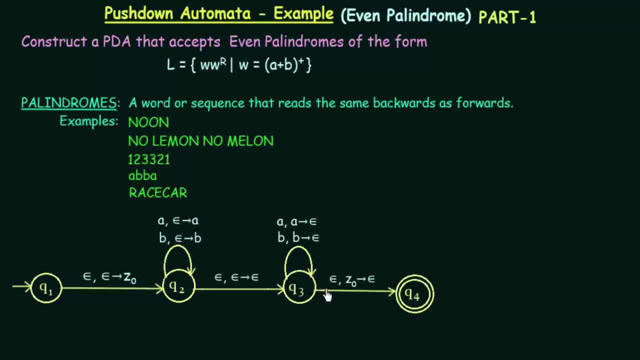 And after that we assume that we have reached the end of the string or our string is finished. And when we reach the end of the string, what we do? We don't read any input symbol, But we check if Z0 is the topmost element of the stack. 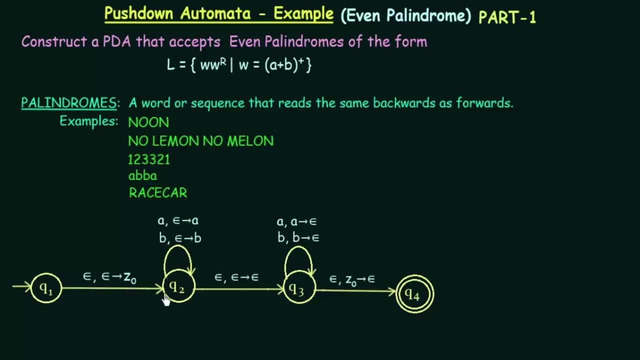 So, if you remember, Z0 was the first element that we pushed. So when everything is popped from the stack, obviously Z0 should be the only thing remaining at the bottom of the stack. opportunity to show you that it is the only element which is remaining at the bottom of the stack. 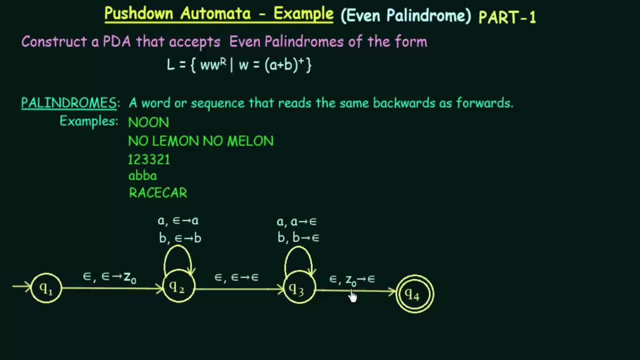 which will be the topmost element in the stack at that point. So check if Z0 is at the topmost and pop it, And then we don't push anything and we reach the final state Q4.. Alright, now let us take an example to make it clear. 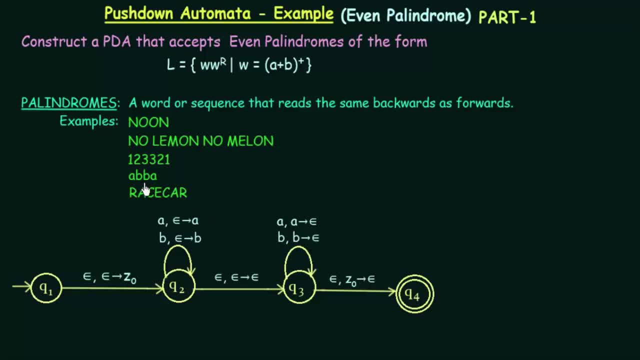 Now let us take this example: A, B, B A. Now let us take this example: A, B, B A. Now let me draw the stack for this. Now, let me draw the stack for this. So here I have drawn the stack. 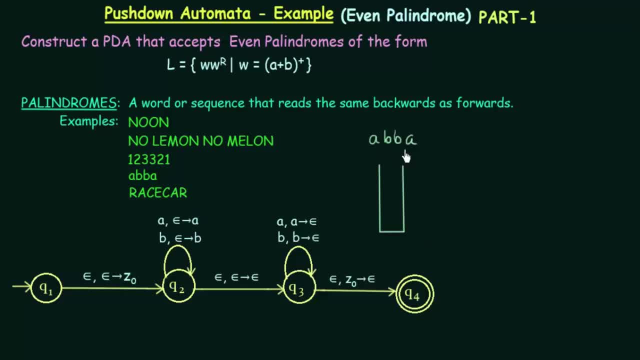 and our input string is A, B, B, A, And we know that this is an even palindrome, because if you read it from here, it is ABBA, and if you read it from blackboard also it is ABBA, And this should actually be accepted by this push-on automata that we have designed. 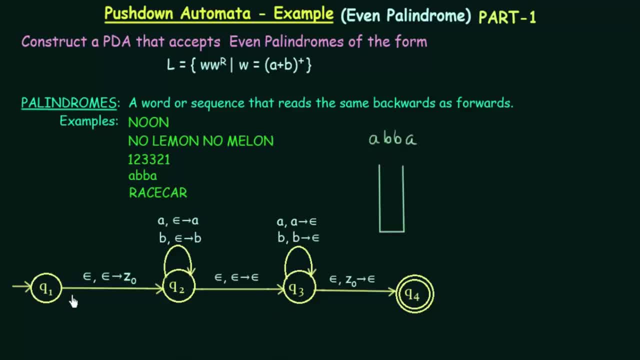 So let's see if it is going to be accepted or not. So first of all, what it is. we start from the starting state Q1, and in Q1 we don't read anything, we don't pop anything, but we push this element Z0 to the stack. 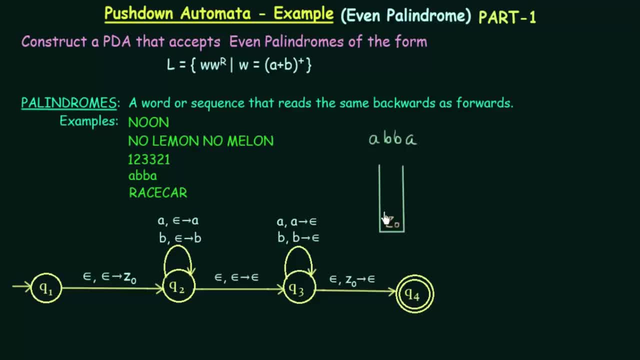 So let me push this Z0 to the stack. So I have inserted this Z0 and now I come to the state Q2 and in the Q2 I get my first input symbol, which is A. Now, when I get the input symbol A, what do I do? I don't pop anything, but I push that A into the stack. 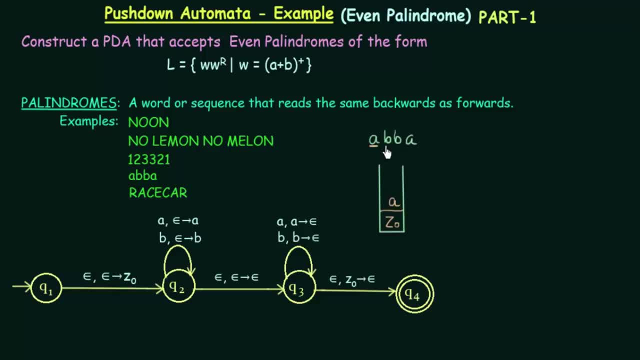 So let me push that A into the stack Now. the next input symbol that I have is B. now I'm still in state Q2, and when I get B in state Q2, what happens? I don't pop anything, but I have to just push that B into my stack. 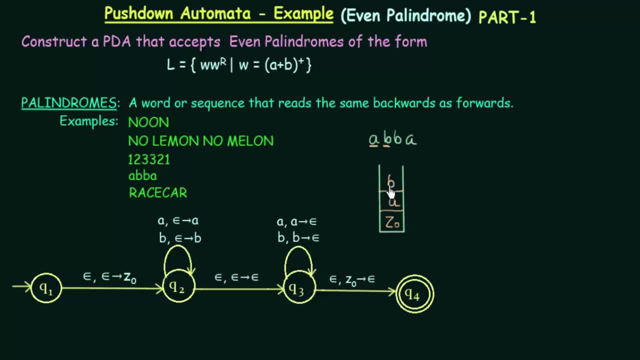 So let me just finish. push this B into my stack now. this is the condition of my stack and if you look here now I have reached the midpoint of my string. this is the middle of my string and when I reach the midpoint I told you we don't read. 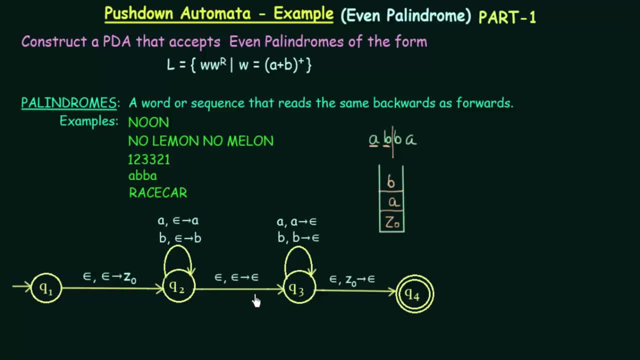 anything. we don't pop anything, we don't push anything, but we directly go to the next state, which is state q3. now in q3, let's see what is the inputs that we get. the next input we get is B over here in state q3. when you get input B, what you 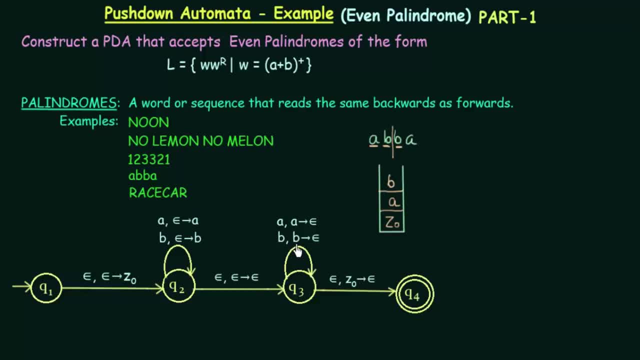 do you check if B is on the top of the stack and then you pop it? now I am checking it here and, yes, I have B on top of my stack. now I have to pop it or delete it. now I have popped it from my stack or I have deleted it from my stack. 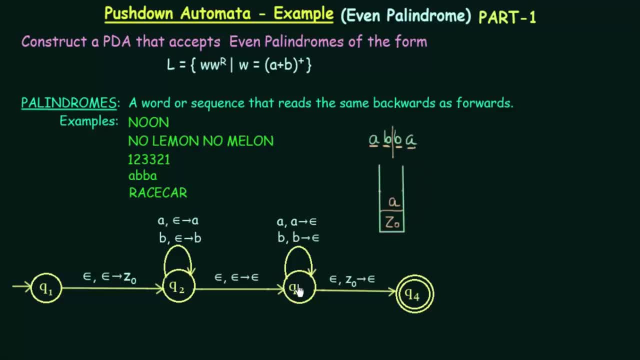 now what is the next input I get? it is a. now I am still in state q3 and in state q3- if I get a, what happens? I should check. If a is on top of the stack, then I have to pop it and we don't have to push anything. 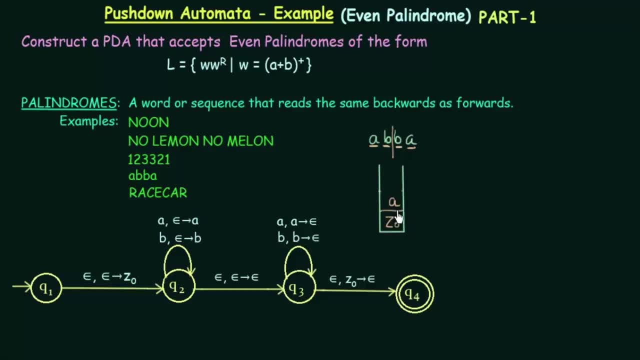 Now let me check. do I have an a on top of my stack? Yes, I do, So I have to pop this a. Now I have popped this a from my stack and the final element that I have is z0. And here I have reached the end of my string. I don't have anything remaining. 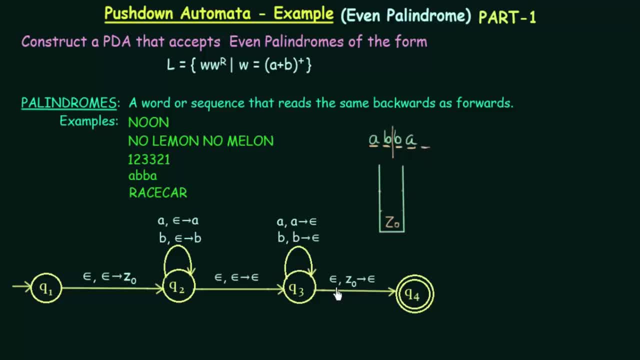 Now, when we reach the end of the string, what do we do? We don't read anything, but we check if z0 is the final element or the topmost element in the stack. Let's check that. Yes, z0 is the topmost element. 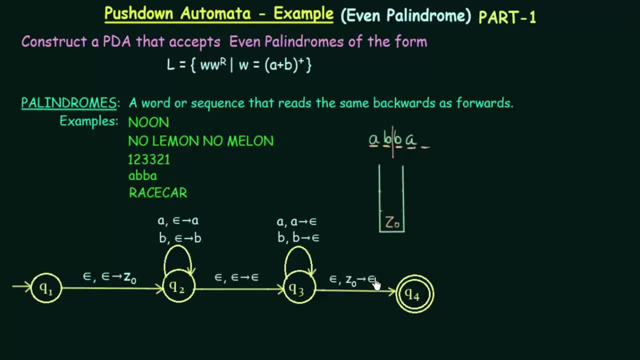 And we can just pop that z0 and we don't have to push anything. So now I have popped that z0 from our stack and now my stack is empty And also we have reached the final state. So since we have reached the final state and also since our stack is empty, this string is accepted. 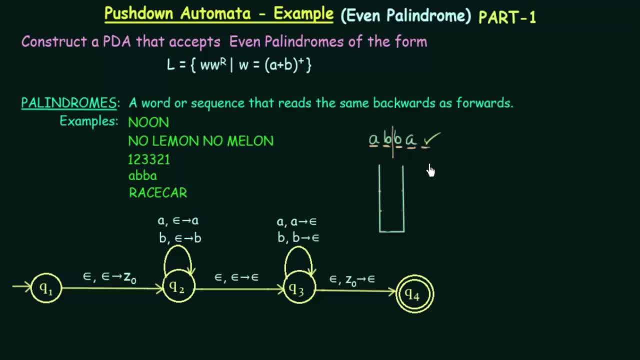 It is an even palindrome. It is accepted. Now let me take another example. Now let's take the string a, b, a b. Now, this string, it is not an even palindrome. Why? Because if I read it from the front, it is a, b, a b. 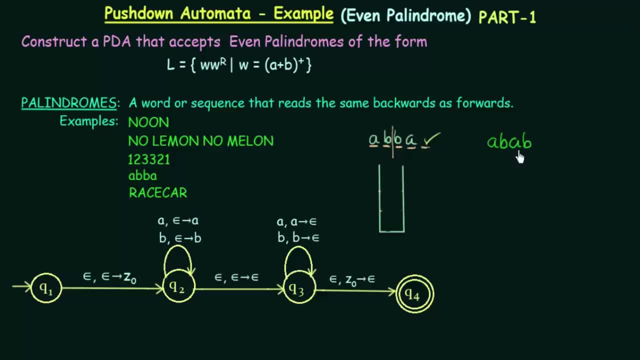 And when I read it from backwards, it is b a, b a. It is not the same forward and backward, So this actually should not be accepted by the PDA that we designed. So let us form the stack for this and see if this string will be accepted or not. 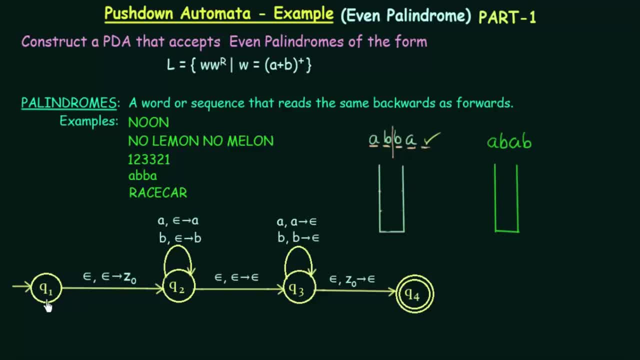 So here I have the stack, I have the stack for this. and then let us come to our starting state q1.. And what do we do in q1? We just push the element z0 to our stack. So let me push z0 to the stack, and then the first input that we get is a. 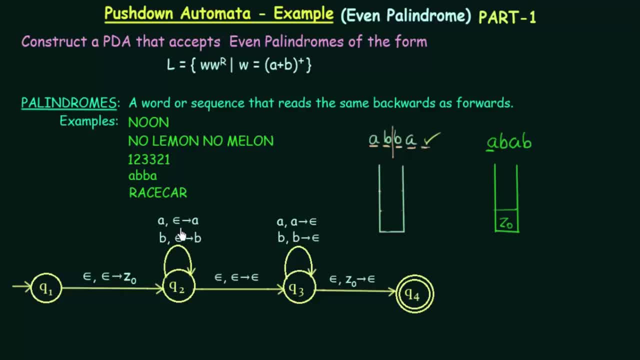 So we are in state q2 and when we get a, what do we do? We don't pop anything, but we just push the a to the stack. We push a to the stack and then we get the next input, which is b. 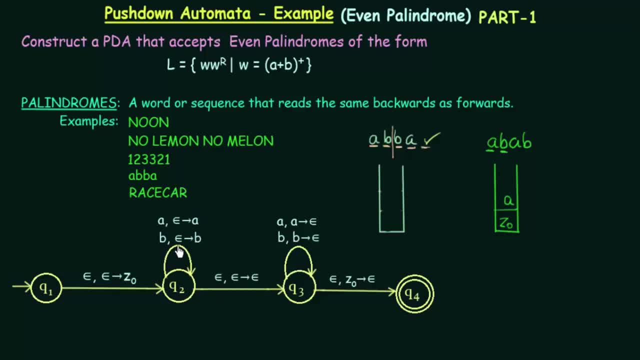 I am still in state q2, and when I get input b I don't pop anything, But I have to push that b to the stack. So I have pushed the b to the stack, Alright. so now here I have reached the midpoint of my string again. 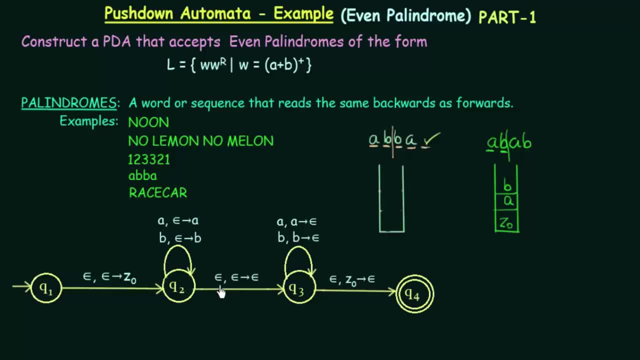 This is the midpoint of my string. So when we reach the midpoint, what do we do? We don't read anything, We don't pop anything, We don't push anything, But we directly go to the next state, which is q3.. 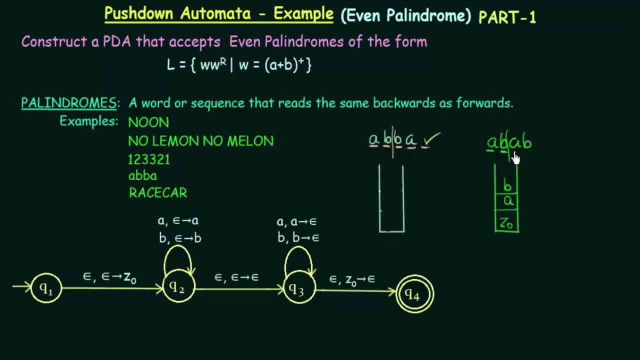 Now in q3, let us see what we are getting. The next input that we are getting is a. So if you get a as an input symbol in q3, you have to check if the topmost element of the stack is a, and then you have to pop it. 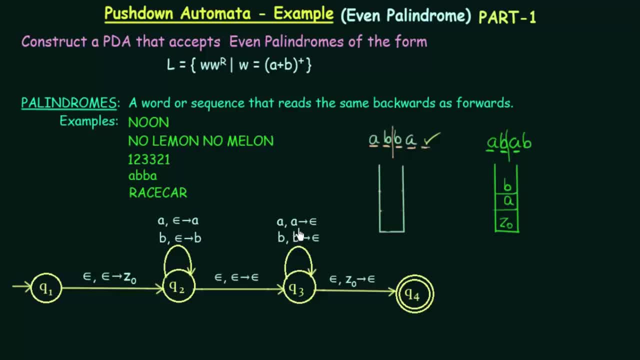 Now I am getting my input a, but when I check whether a is the topmost element of my stack, no, it is not. The topmost element of my stack is b, It is not a. So this state cannot proceed and there is nowhere this state can go and hence it cannot reach the final state. 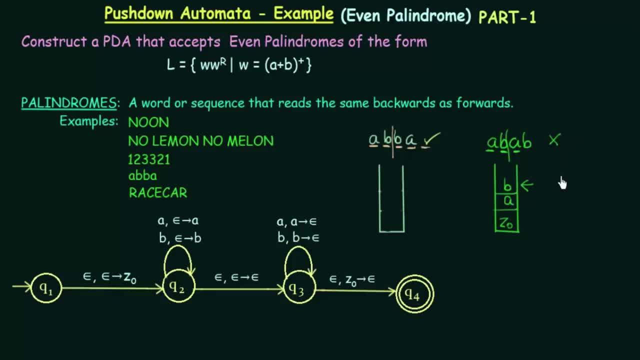 So this string will not be accepted. So this is how you design a string. This is how you design a push down automata that accepts even palindromes of this form. Now, if you have been listening carefully, there must be some doubts that you must be having. 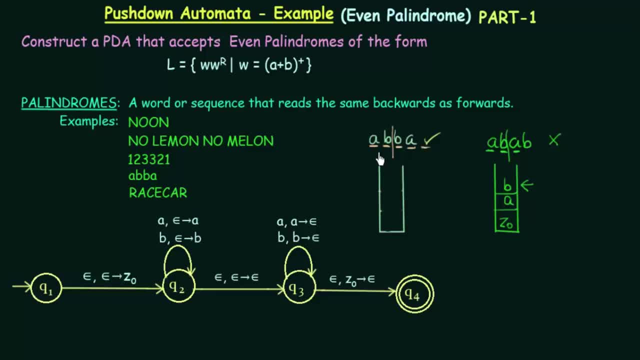 The first doubt that you must be having is that I told you that when you reach the midpoint, we don't read anything, we don't pop anything, but we go to the next state. So in the first half we just push the elements to the stack and then, when we reach the midpoint, 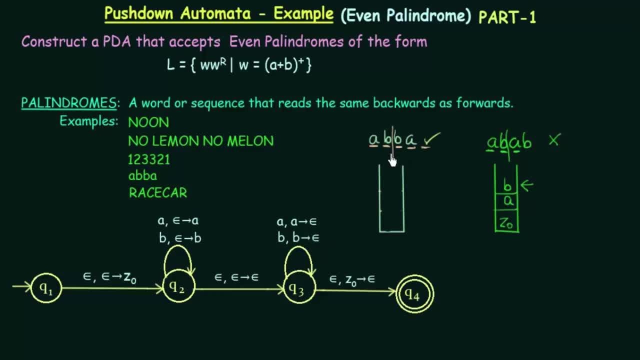 we started popping the elements, But how do we really know when we have reached the midpoint of our stack? There is nothing here to specify that I have reached the midpoint of the stack. So how do we know that I have reached the midpoint of the stack or not? 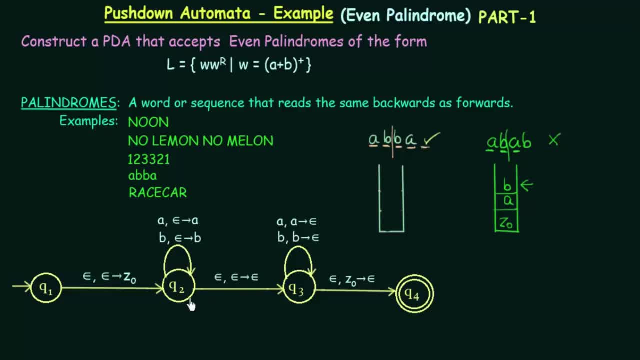 And how do I know when should I take this transition from state Q2 to Q3?? This is one question you must be having. So this question I will be answering in the next lecture and I will be explaining it in a very detailed way. 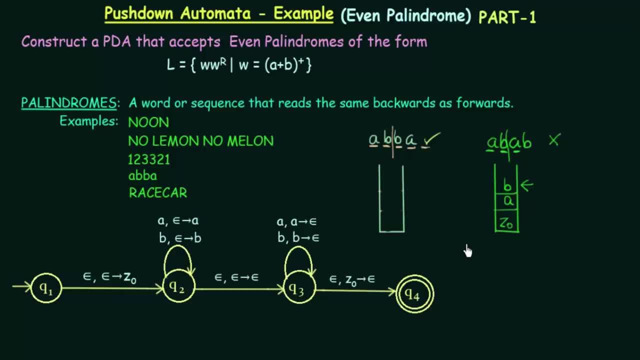 But in the meanwhile, if you have any questions, please do not hesitate to ask in the comment section. And if you have any idea how this is done, I request you to drop your idea in the comment section And in the next lecture you can check out whether it is correct or not.